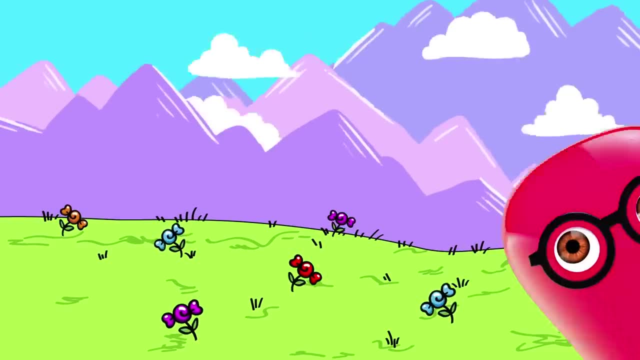 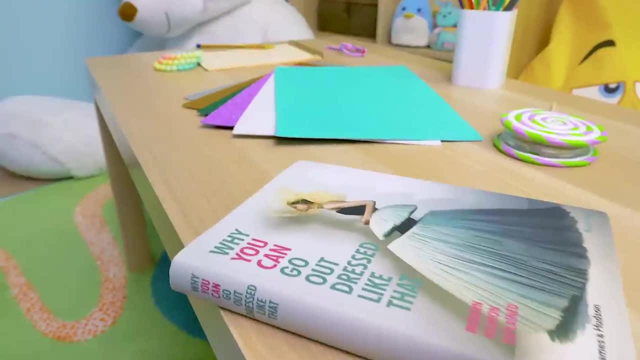 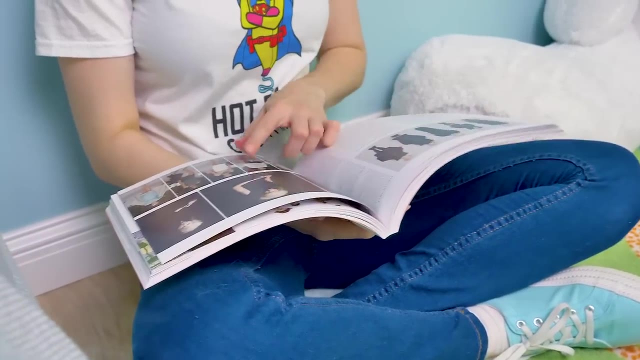 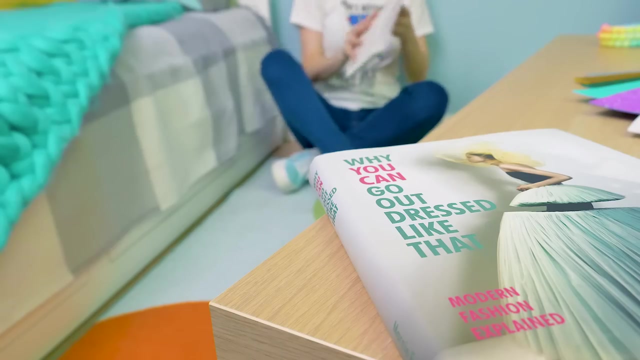 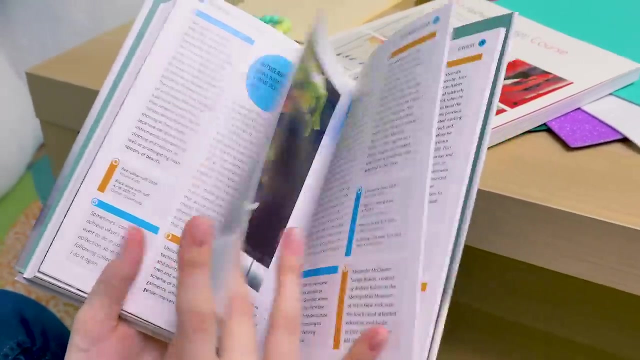 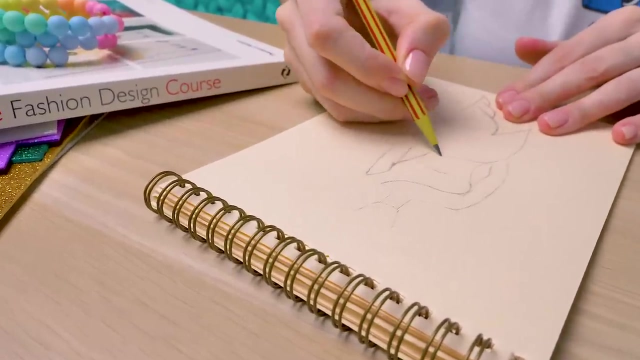 Ah, these are so beautiful and unusual. I'd love my outfits to take part in a fashion show one day. Ah, but to achieve this I need to study a lot and learn to create new outfits. Fashion design is amazing. I'm glad I started to study it. 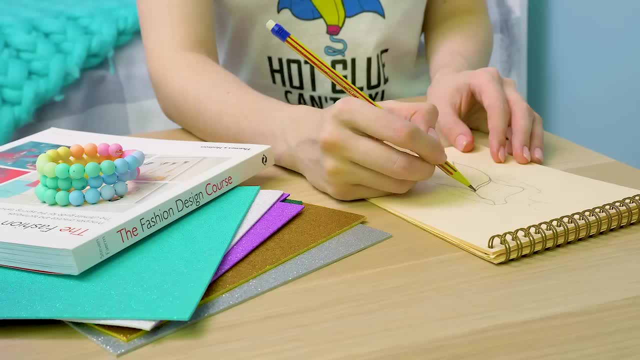 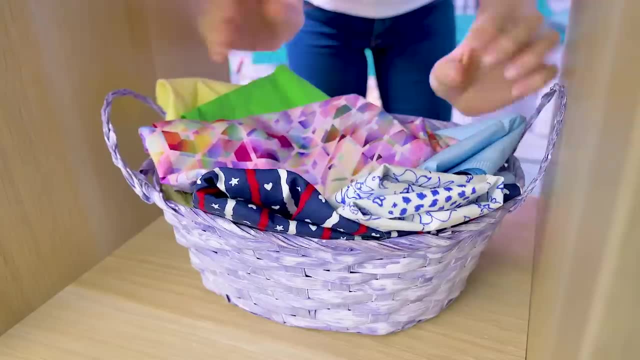 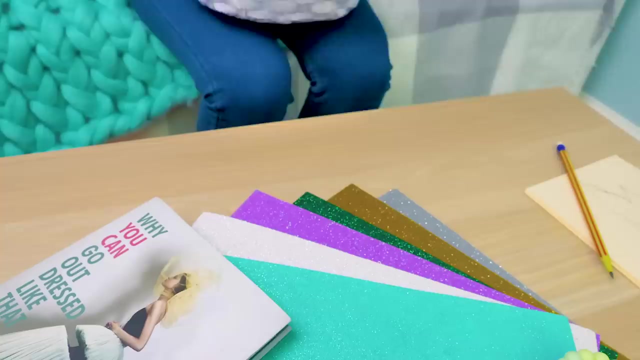 Hey guys, have you ever created your own outfits? Write in the comments, Right, and I need to practice. Drawing is good, but I need to move on to real-life outfits to understand how they'd look in reality. Huh, I don't have enough fabric, Can't do much with these, And who will be my model? 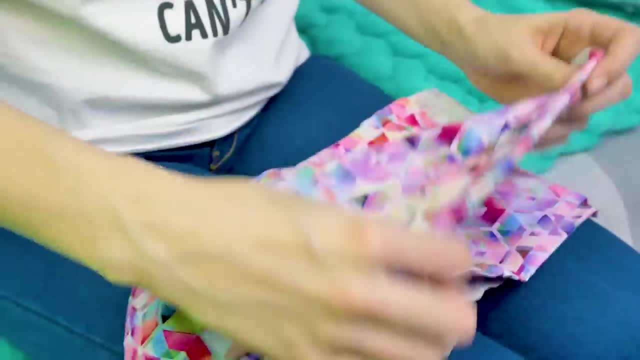 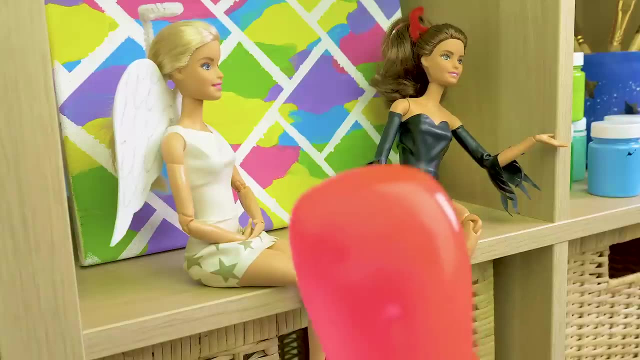 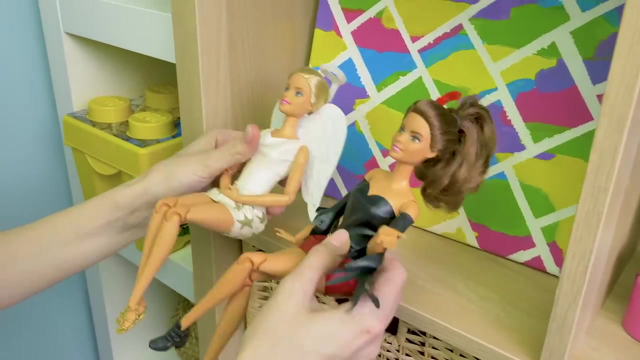 I will. Oh, Sammy, thank you so much, but I want to make dresses. Oh, I think I'll skip dresses. Oh, use your Barbie dolls. Are they sitting here for nothing? Barbie dolls? Oh, that's a wonderful idea. Thank you, Sammy. 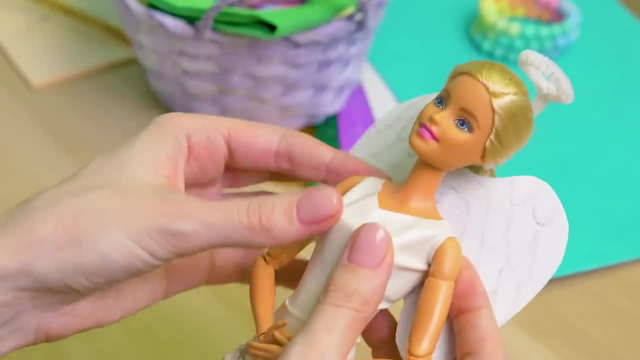 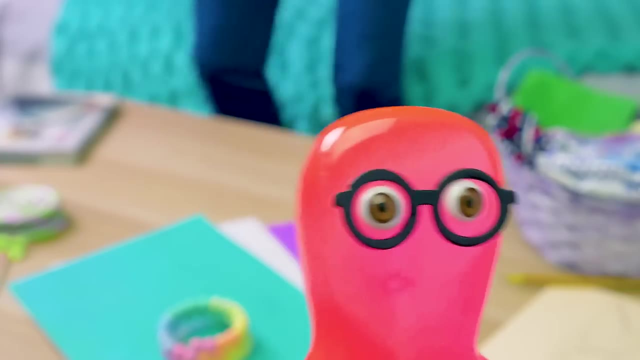 You're welcome. I won't only use dolls as models. I'll use Samantha's idea to use balloons. Do you remember the video where Samantha and I made these outfits? Give a thumbs up if you did. Susie, wait for me. 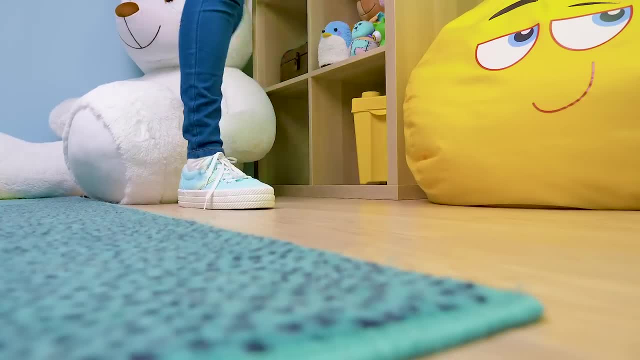 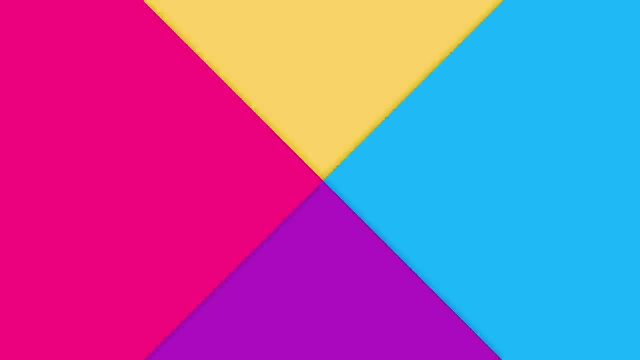 Sam, do you remember where the box of balloons is? There were a lot of them left. Yes, yes, I'll go get it. Oh, and I'll get everything ready. Hi everyone, We're going to hold a workshop on how to create simple doll outfits. 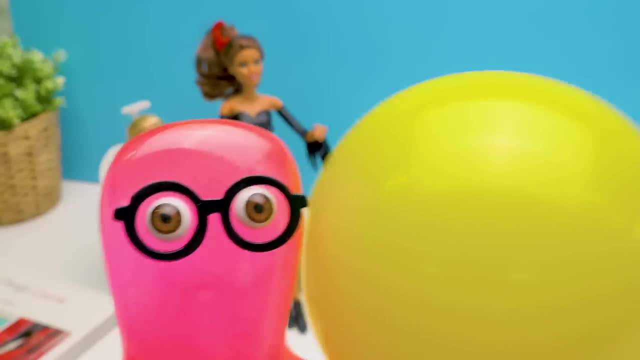 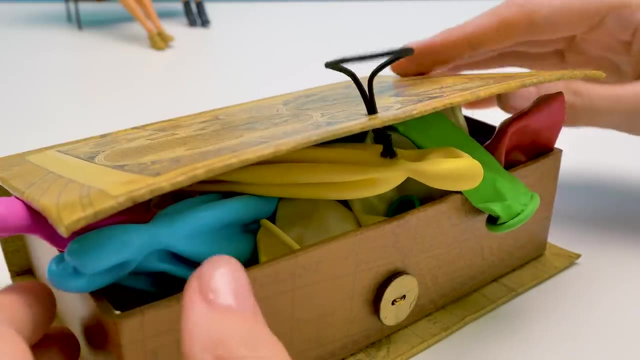 And for me it'll be fashion-oriented, And for me, balloon fun. Oopsie Can't do without fun. Here's your balloon supply- Great Sammy thanks. And for today's outfits we'll only need colorful balloons of different types and scissors. 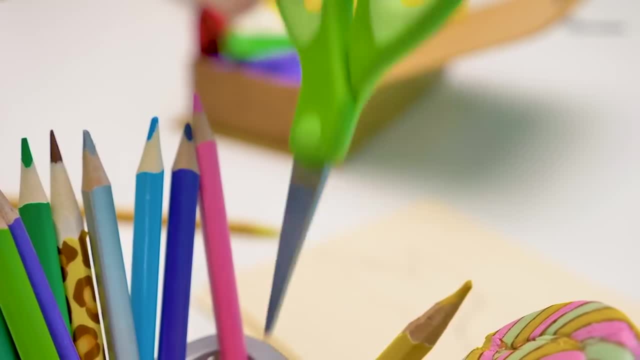 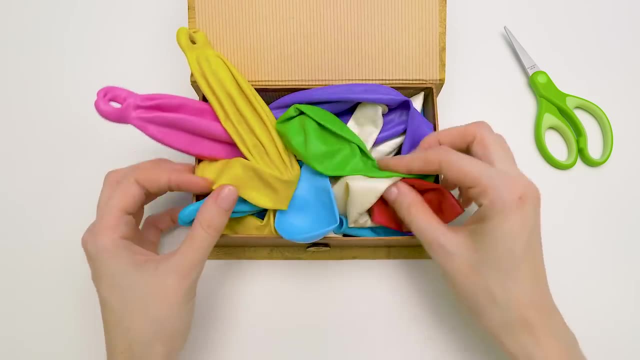 Don't forget to be careful with scissors. And what will you start with? Hmm, let's see what we have here. Aha, These two balloons complement each other. I'll make a top from the blue balloon And a top from the blue balloon. 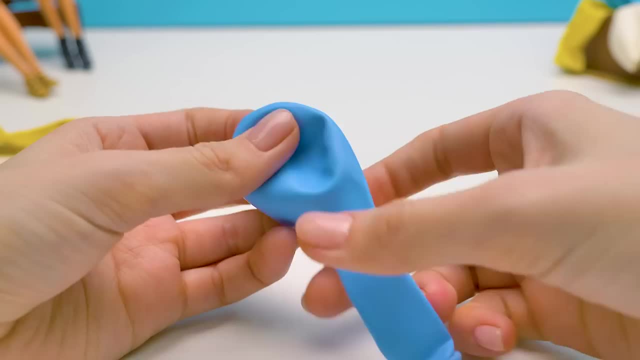 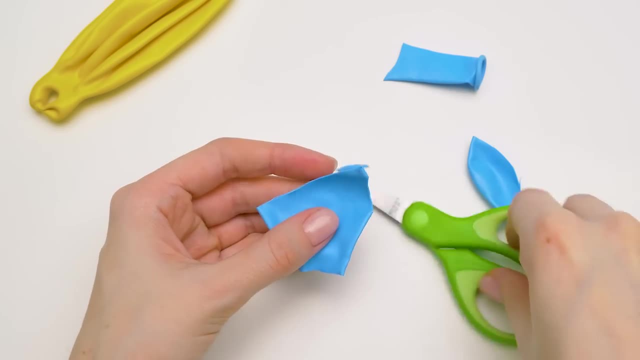 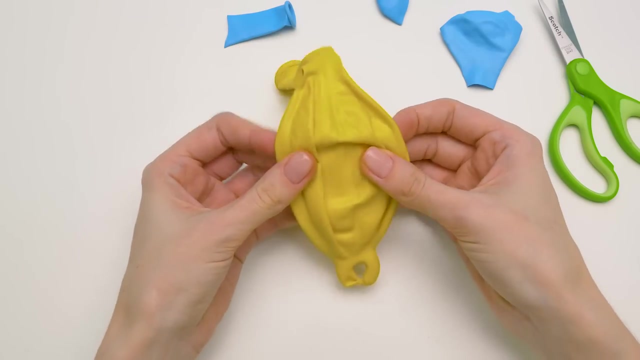 Right, This is the opening for the arms. And here's our stylish top. And here's our stylish top. Let's make a cool skirt to match it. This balloon will make a wonderful pleated skirt. This balloon will make a wonderful pleated skirt. 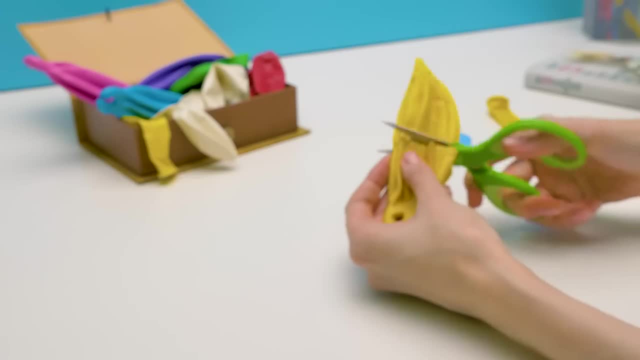 To make it, we'll need to cut off the top and the bottom part of the balloon. To make it, we'll need to cut off the top and the bottom part of the balloon. I also made something for myself from the balloon. That's stylish. 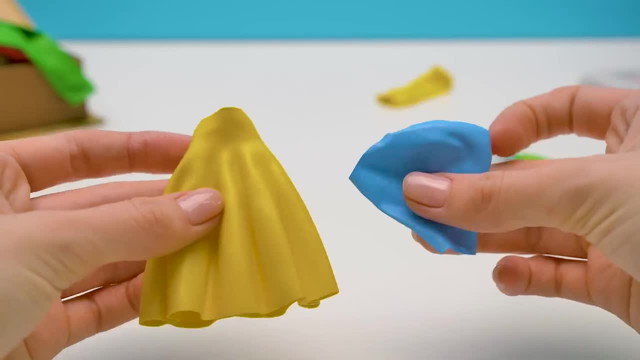 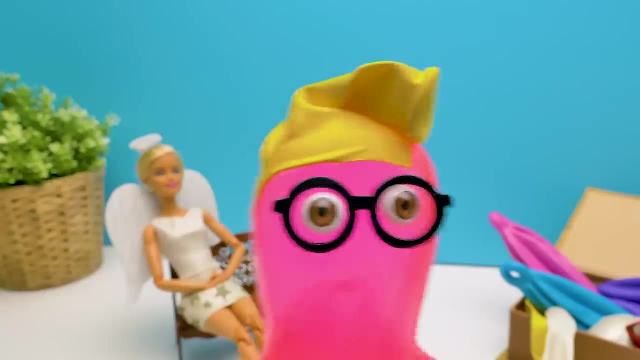 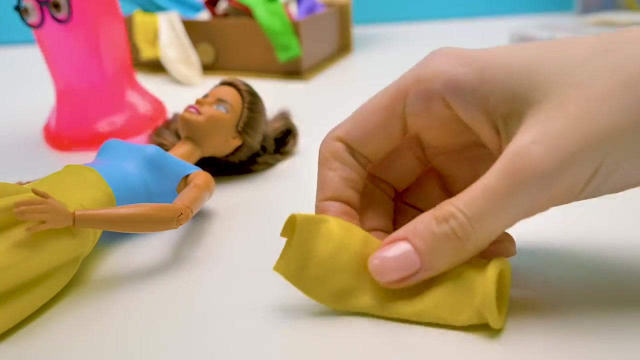 Yeah, Time to try the outfit on. Come here, beautiful doll, And hop Sue, you forgot an important detail. What, Sammy? An accessory? I keep hinting. Oh right, right, I'll use the remainder of the yellow balloon to make a hairband. 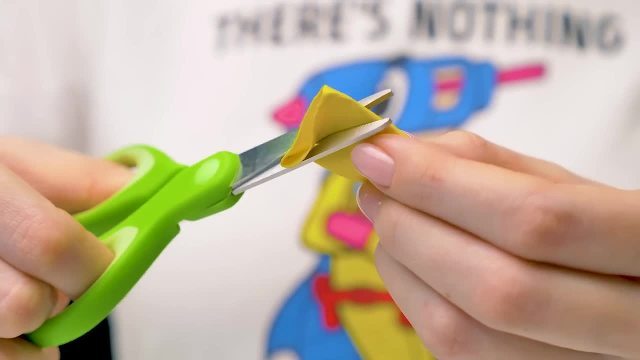 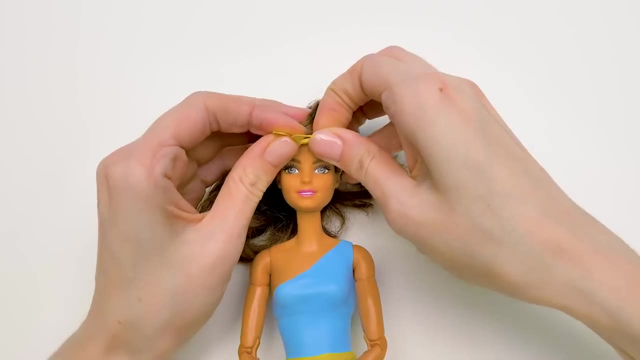 I'll cut off this ring And a piece of the balloon. Right, I need to shape it Great. Now let's tie this piece around the ring. Done, Let's put it on Carefully not to tear it. Great. 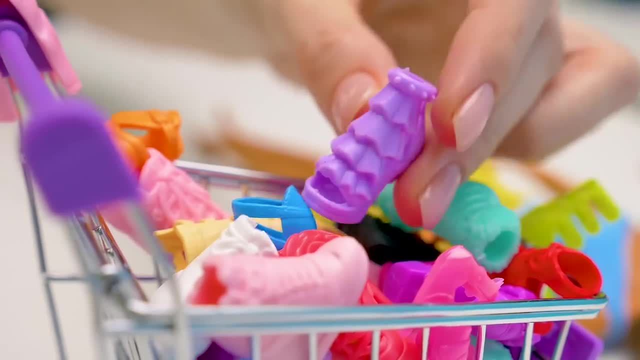 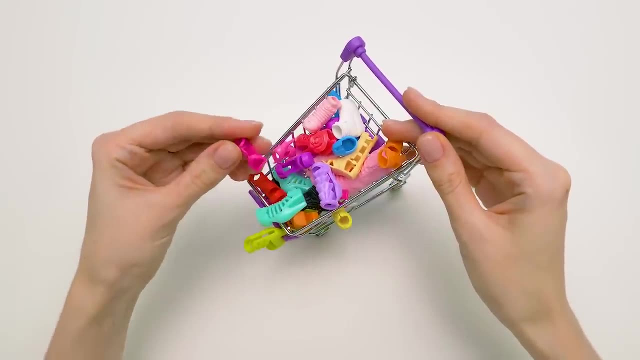 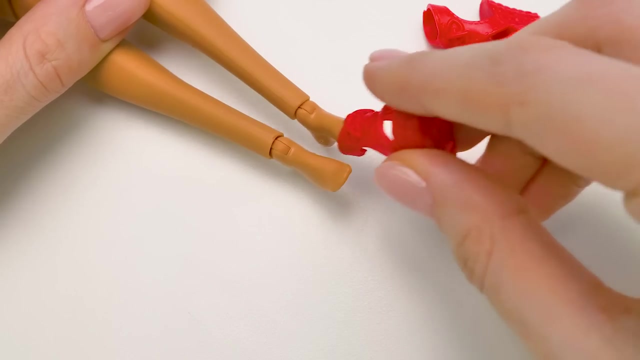 And we also need Shoes. Wow, Sammy, you can read my mind. I know a thing or two about style. Wonderful, Right, let's see. And maybe, Aha, Yes, these, Let's try them on One and two. 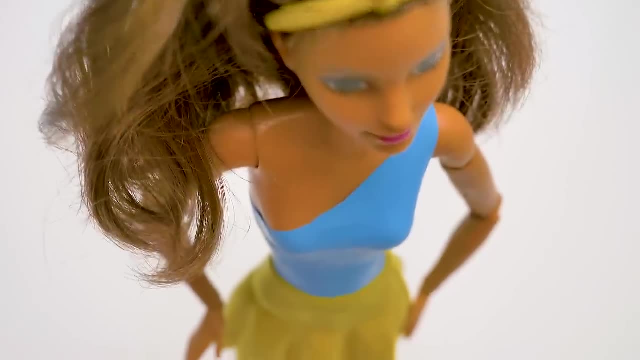 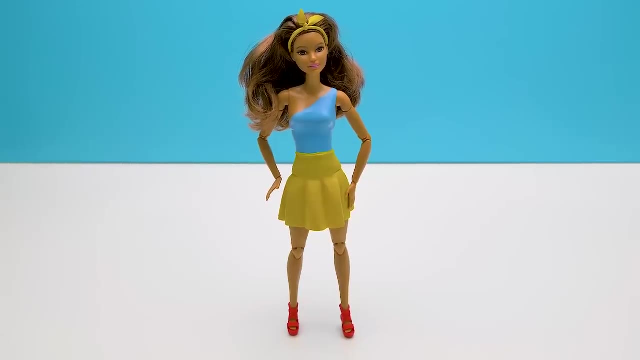 Now it's done. Next I'll make a dress. It'll be fashionable: purple. A ruffled balloon will be great for that. I only need to cut it on the top and at the bottom There. Come here, You'll have to part with this beautiful angel costume. 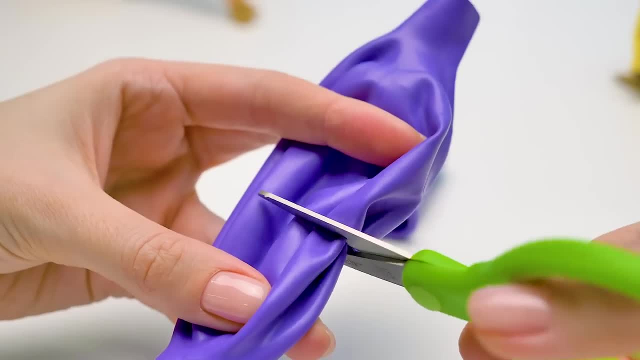 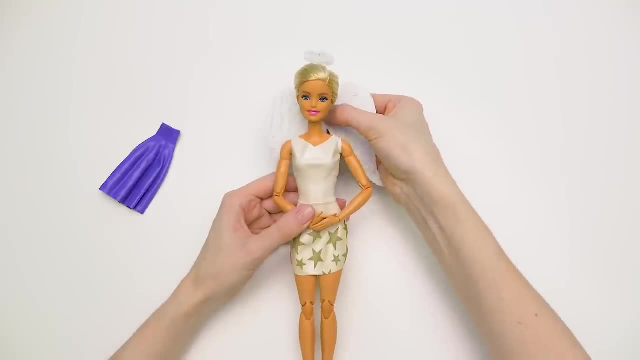 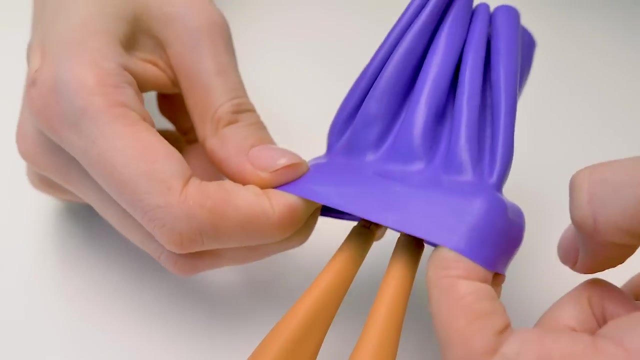 But there's an amazing dress waiting for you. Let's try it on, And Yes, And Yes, And Yes, Let's try it on carefully. Maybe putting a balloon on isn't very fast, But it looks elegant Done. 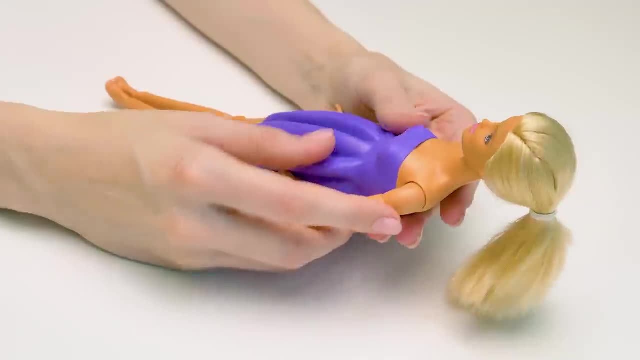 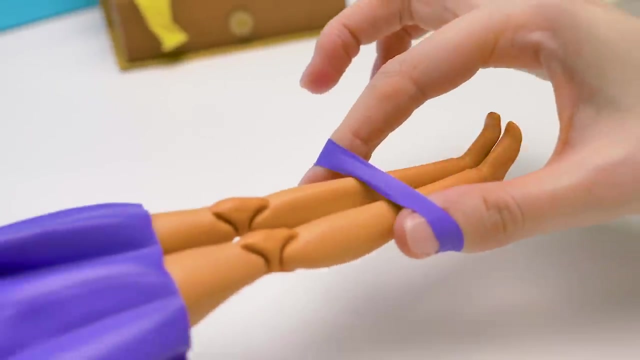 Only Too simple. Yes, let's add a small detail. I'll cut two pieces of a balloon from the narrow part And two. I'll put this piece on the top of the upper part of the dress. Nice and slow, And I'll adjust it. 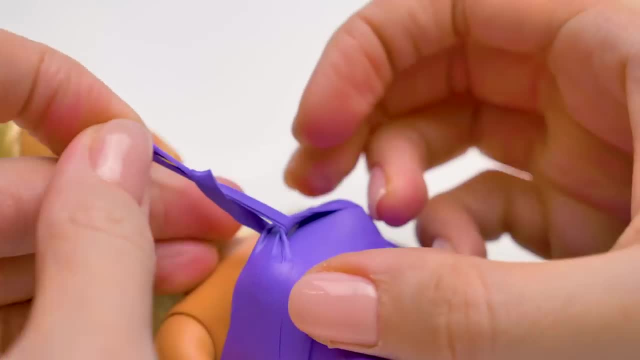 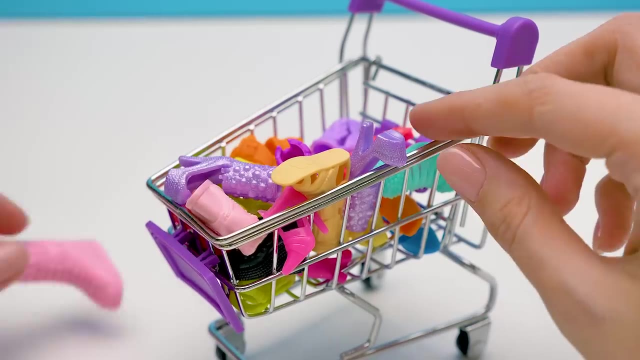 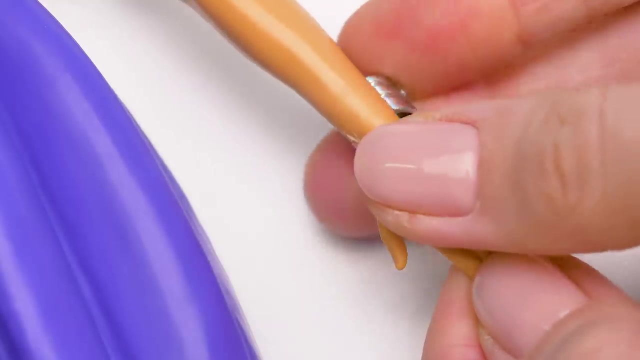 Right, And this narrow piece will go through the wide one And over the head. Let's smooth it all out And voila Time to add some accessories. These shoes will highlight the festive mood of the dress. And a bracelet. And a bracelet. 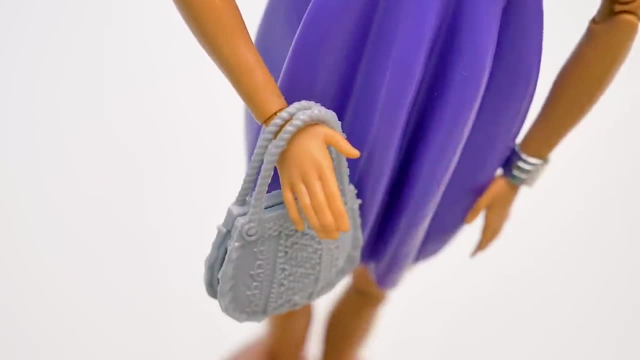 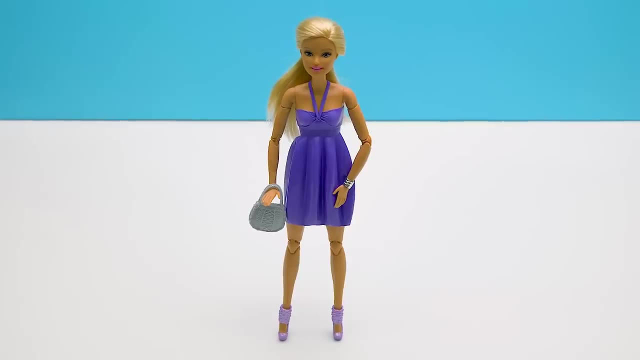 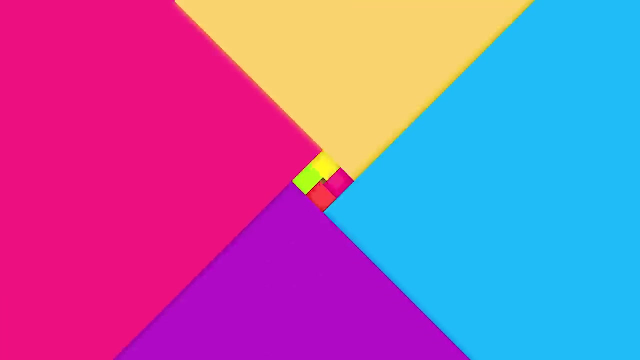 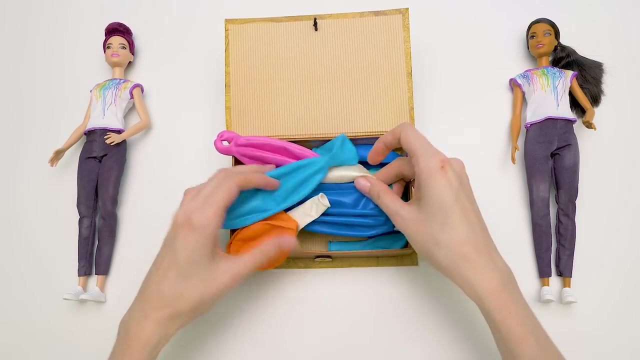 And a bracelet And a handbag Done From the heaven straight to the ball. Allow me, mademoiselle. And these two beauties also want new outfits. New outfits, No problem, I've got so many balloons left. 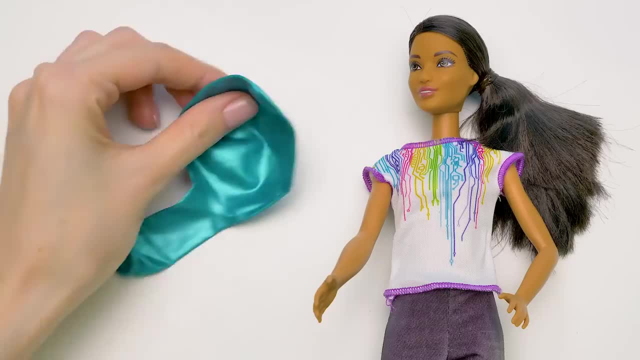 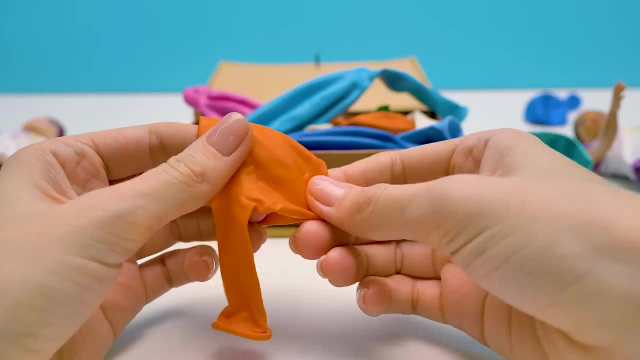 Right, let's see which colors will suit each of you. Hmm, this is a wonderful turquoise color For you, And for you this one, Ah no, Oh yes. So bright and sunny And this clear white to accompany it. 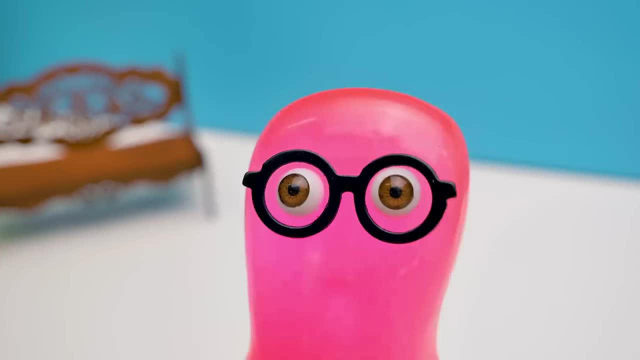 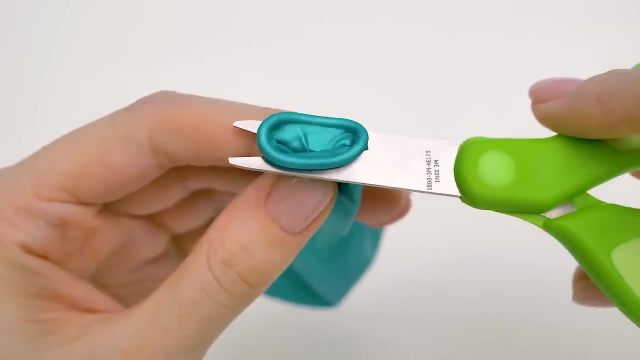 Let's go Go on and I'll select some accessories for it. All right, I trust you with this important task. Thank you, Susan, I won't let you down. Right To make a strict sheath dress, I need to cut off the ring. 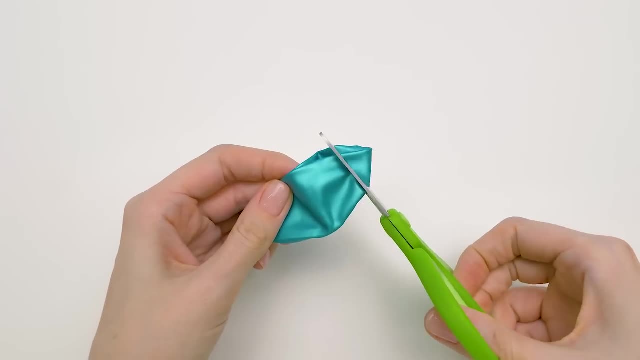 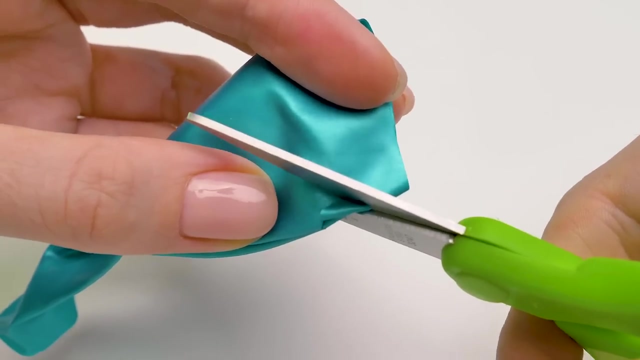 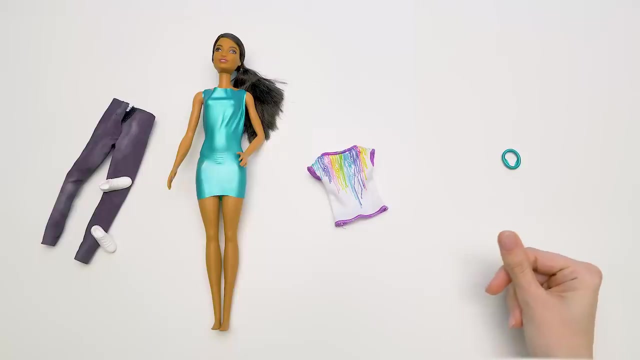 We'll need it later. And the top of the balloon, Just like this. Okay, Now let's make holes for the arms. I'll cut out neat triangles. It's better to go slowly here. These are our openings. Time to put the dress on. 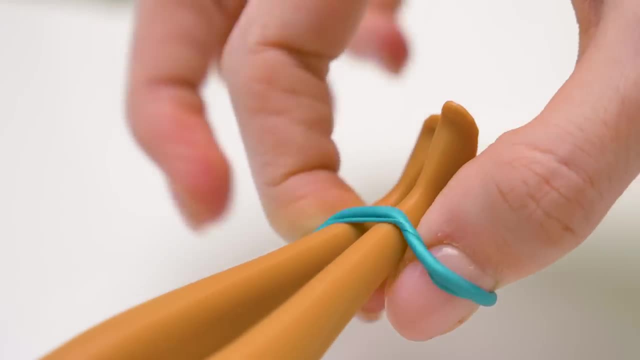 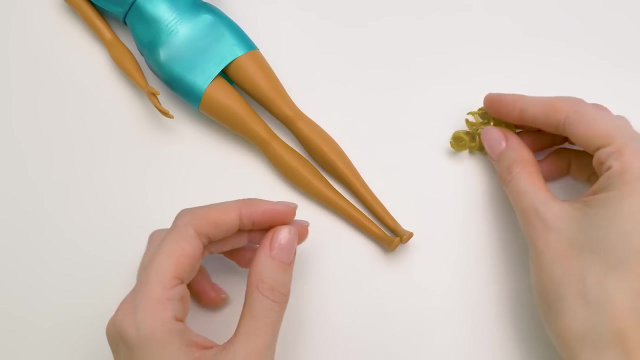 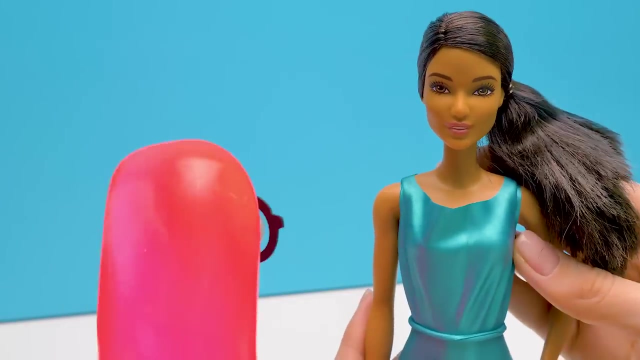 Now we only need to decorate the dress with a cute belt Like this. Take these shoes. Oh wonderful, Sam, I couldn't have selected better shoes myself. One and two And done. Beautiful, A very busy, like elegant lady. 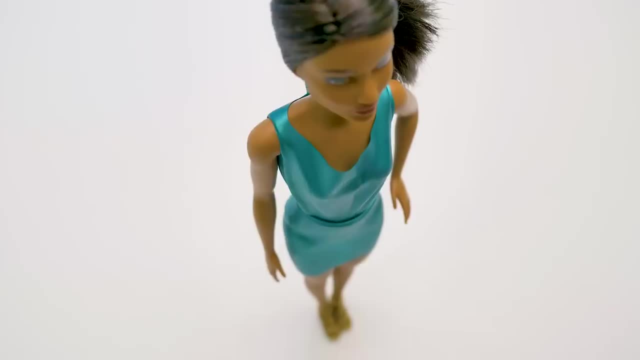 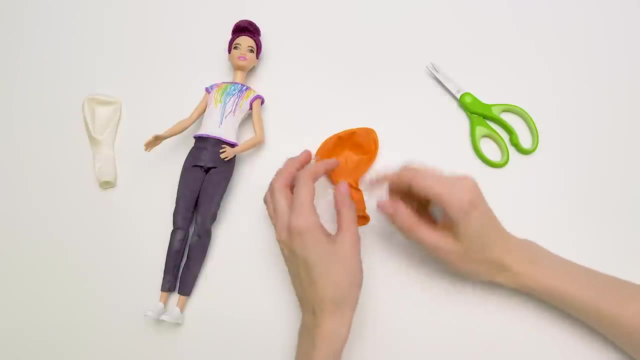 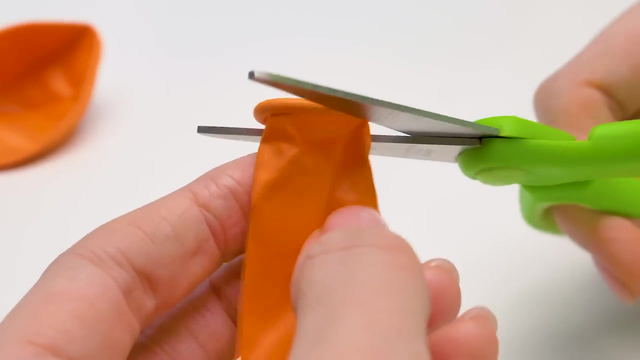 I'm glad you like it, So let's dress you up as well. This wonderful sunny orange balloon will make a wonderful top. I'll cut it off here At the top And at the bottom To make a narrow strip, But not too narrow.